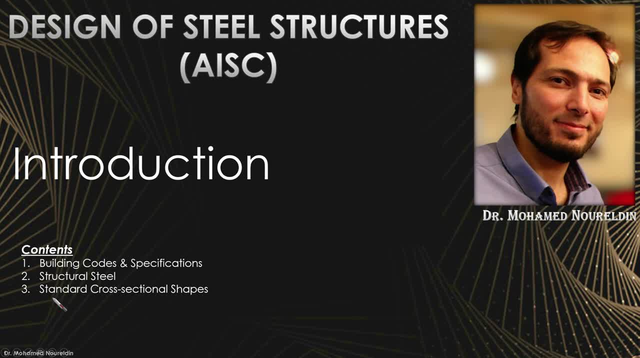 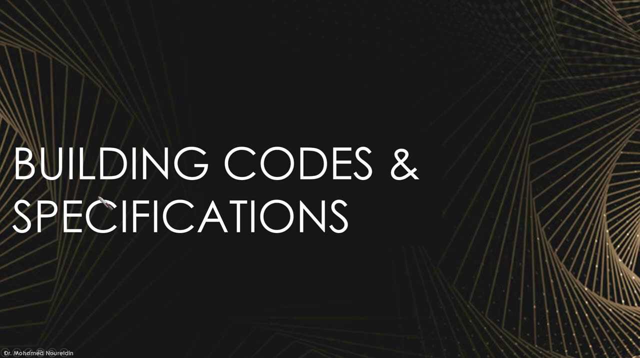 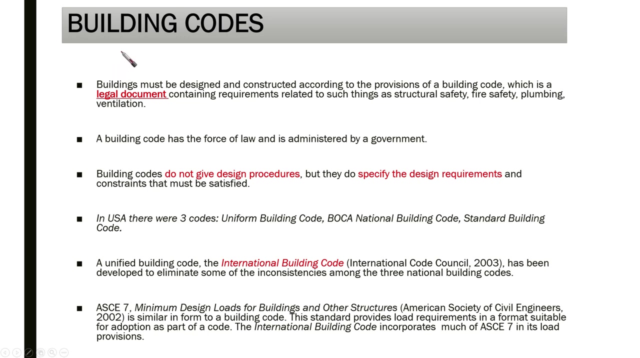 then, after that, I'm going to give an exposure regarding standard cross-sectional shapes that is going to be used in our design in general. Okay, let's go directly to the first point, which is going to be, as I said, building codes and specifications. So, first of all, we want to understand what is the meaning of 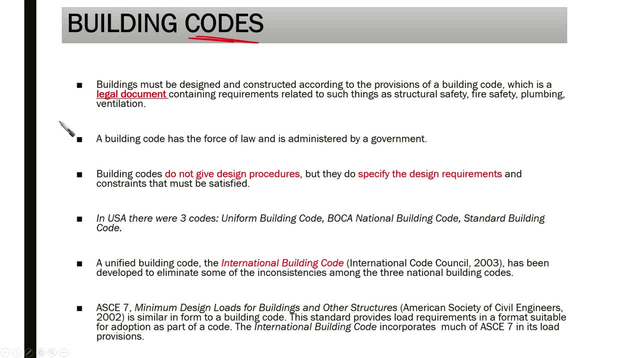 building codes from different points or based on different points. So, first of all, let me go with this hint, which is an important hint, to understand the legal, or from the legal point of view, what or building codes. Okay, buildings must be designed and constructed according to provisions of building. 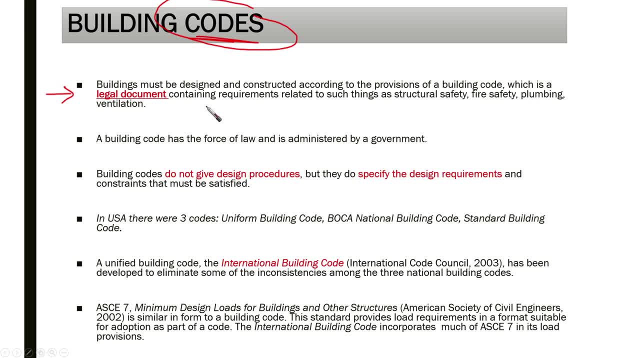 codes, which is a legal document containing requirements related to such things as structure safety, fire safety, plumbing, ventilation. So the key word here is legal document. So it is considered to be a legal document. A building code has the force of law and is administered by. 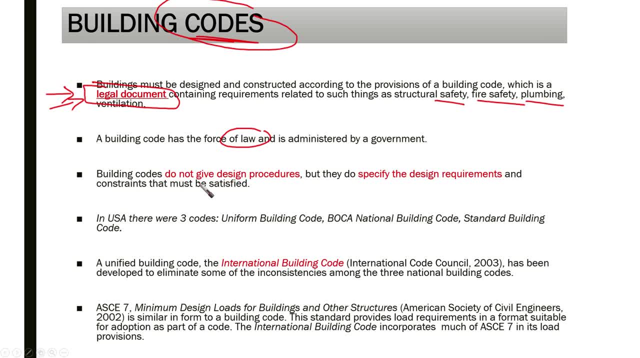 the government Building codes does not, or building codes do not give design procedures. This is an important issue here which is different than other things. It does not. or building codes do not give design procedures, but they specify the design requirement. Just they are giving some requirements. 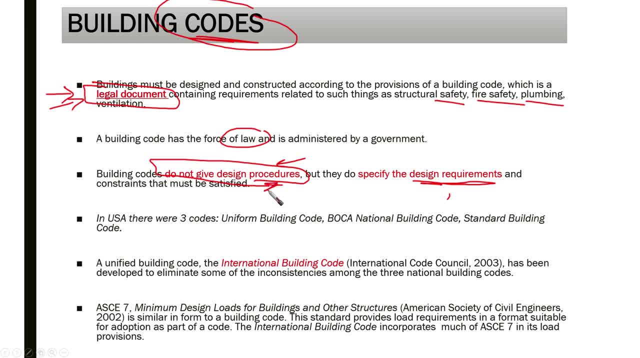 for the design, but they do not prescribe or give any design procedures and constraints that must be satisfied. So they are providing design requirements and constraints that must be satisfied. So they are providing design requirements and constraints that must be satisfied. And the US? there is three different. 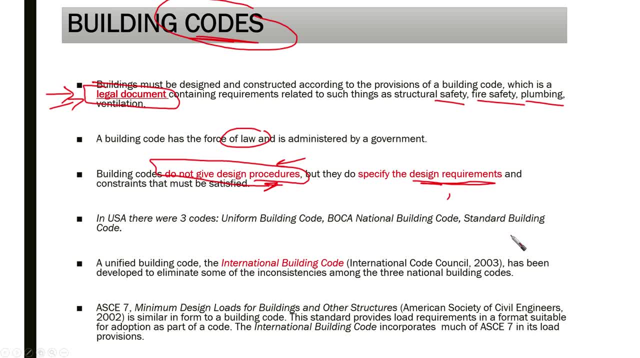 codes: uniform building code, national building code and standard building code. A unified building code, which we call it the international building code, international code council okay- has been developed to eliminate some of the inconsistencies among the three national building codes There is. 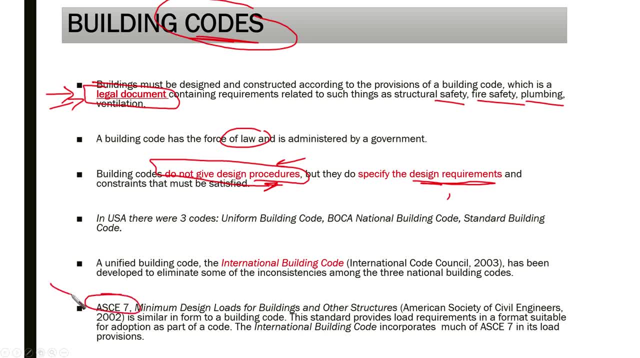 an important we can say code. it is loading code which is a building code. It is a building code. ASCE- American Society for Civil Engineers 7, we call it the minimum design loads for buildings and other structures. okay is similar in form to a building code. This standard provides load requirements in a 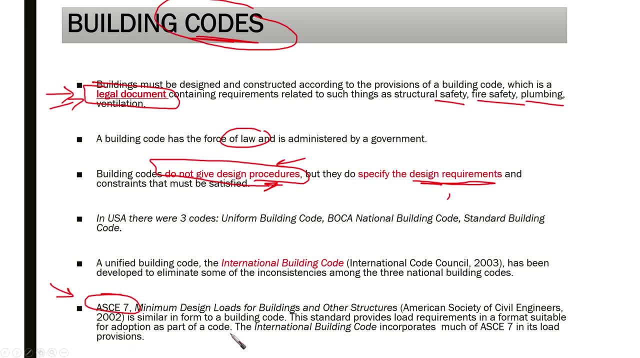 format suitable for adaption as part of a code. The international building code incorporates much of ASCE 7 and its load provisions. Whenever it comes to the load provisions, you are going to find that ibc or the international building code is making reference to asce7. so we need to know. 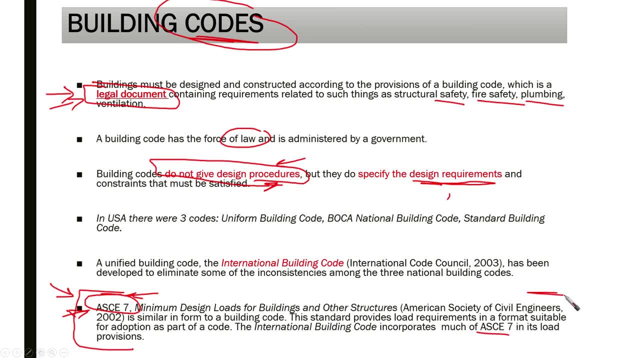 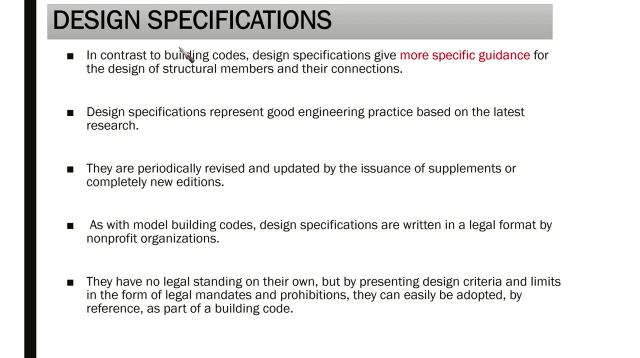 or to have an exposure to it and to be familiar with this ase7, because it is going to be very important for us, especially whenever we are talking about load combinations. okay, let's go now and understand what is the meaning of specification, design specification, so in 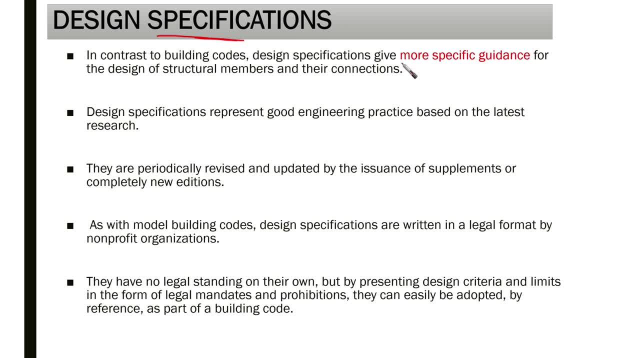 contrast to building codes, design specifications give more specific guidance. okay, so it is going to give you more details for the design of structural members and their connections. design specifications represent good engineering practice based on the latest research, and they are periodically revised and updated by the issuance of supplements. 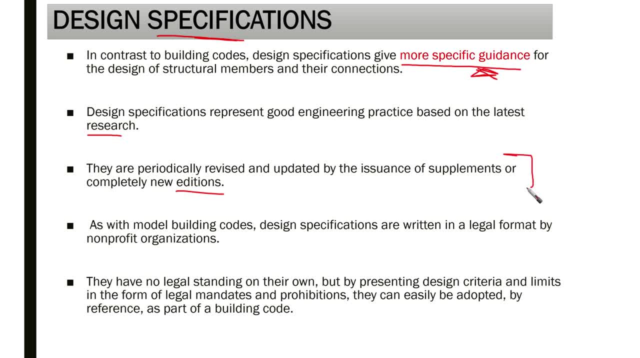 or the implementation of the design specifications. so, in contrast to building codes, design specifications or completely new additions, as you can see, if we're talking about a, i, s, c, so we're going to find that different editions are always provided and it is periodically revised and different issues are issued every almost three years or more. okay, as with model building codes, 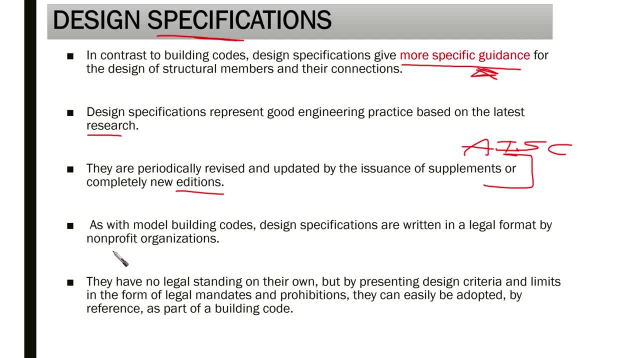 design specifications are written in a legal format by non-profit organizations. they have no legal standing on their own. okay, so remember that they do not have any kind of legal standing. so this is an important issue. actually, whenever that you are designing or reviewing a building or a project, it is important to keep in your mind that it is only like giving you. 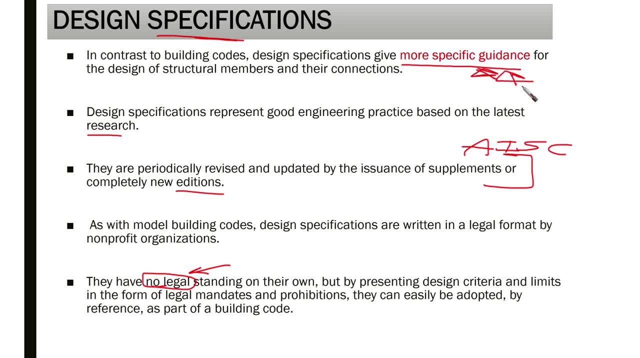 specific guidance, but it has no legal obligation upon you. okay, so that's the the point. so they have no legal standing on their own, but they but by presenting design criteria and limits in the form of legal mandates and prohibitions, they can easily be adopted by reference as part of the building. 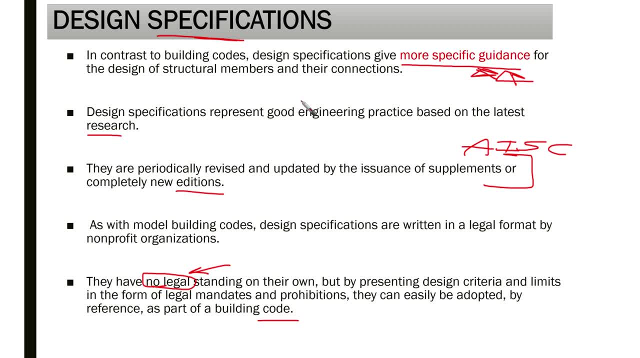 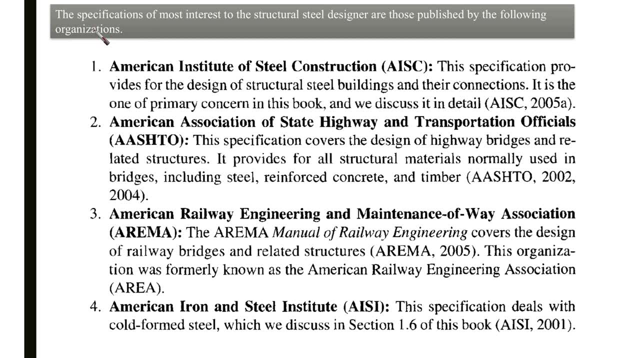 code. okay, so this is the difference between the building code and specifications. now let's go and see what are the specifications of most interest to the structural steel designer are those published by the following organization: we have actually like important four different structural steel. we can say specifications that very important for the structural steel designer. 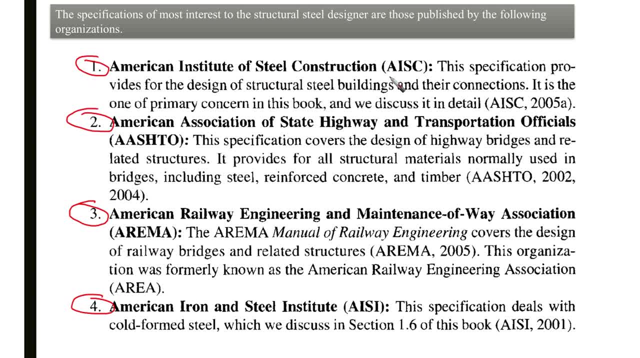 in general. first of all, the american institute of steel construction. we call it a i s c, a i s c. this specification provides more, provides for the design of structural steel buildings and their connections. it is the one of primary concern in our, in our videos, in our course here. the second specification: we call it american association of. 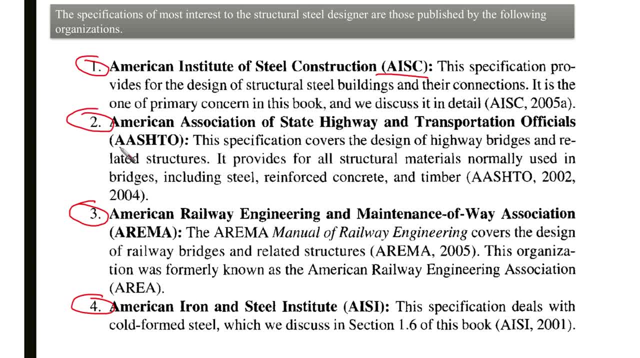 state highway and transportation officials. we call it for short ash 2.. this specification covers the design of highway bridges and related structures. it provides for all structural materials normally used in bridges, including steel, reinforced create, rein� reinforced concrete and timber. The third specification is the American Railway Engineering and Maintenance of Way Association. 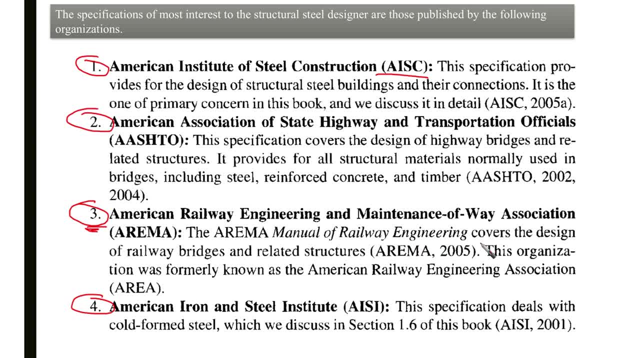 The ARIMA Manual of Railway Engineering covers the design of railway bridges and related structures. This organization was formerly known as the American Railway Engineering Association. And the last specification, number four, which is important for us, is the American Iron and Steel Institute. 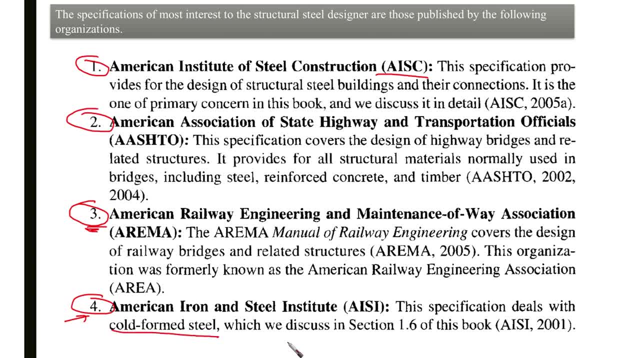 This specification deals with cold-formed steel, which we are going to discuss- Actually, we are not going to discuss in our course, but it is related to the textbook that we are using. So, in general, what is important for us? We are going to highly concentrate on AISC. 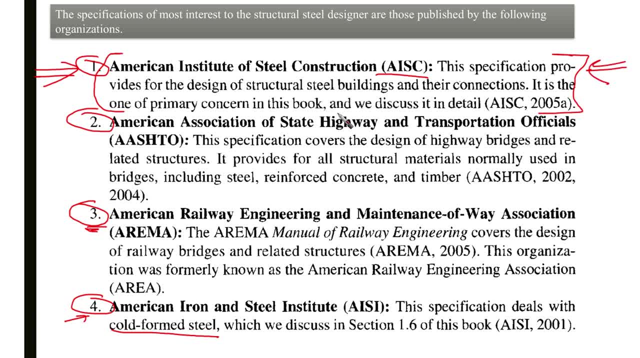 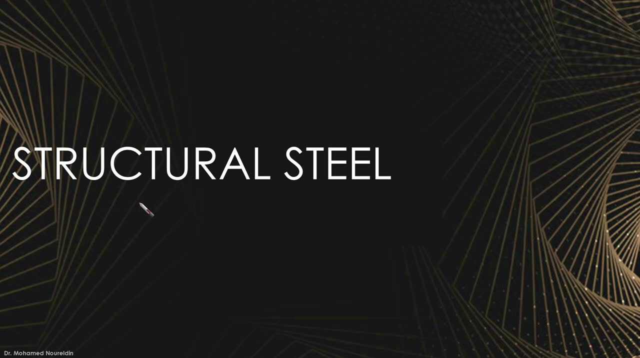 This is our main concern in our code. We are not going to discuss about or refer to AASHTO or ARIMA. Maybe to some extent we can find this cold form, but actually it is not the main concern of our course. Now let's go to the structure steel and try to understand more about the types of structure. 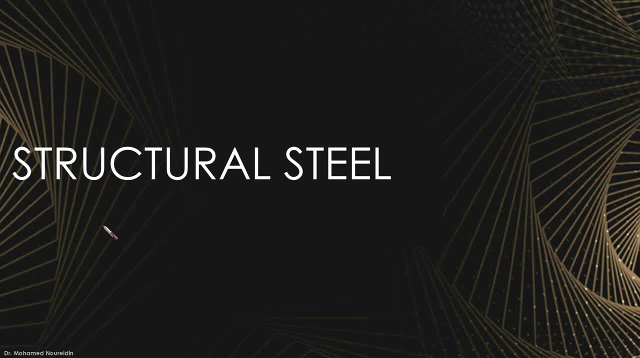 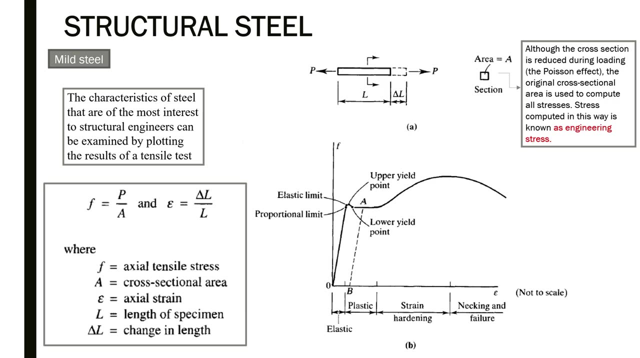 steel. We have commonly different types of steel. We are going to know some of them today. So we have first We have here mild steel. This is the first type of structure steel that we are going to face and we are going to use in our course. 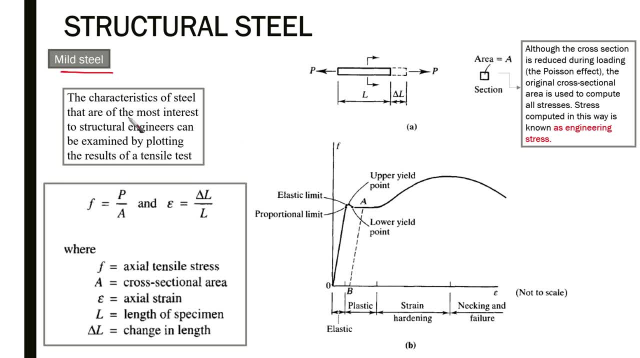 So the characteristics of steel that are of the most interest to structure engineers can be examined by plotting results of the tensile test Whenever that we have a specimen and we put it under tensile test, So we have tensile loading, as you can see here. 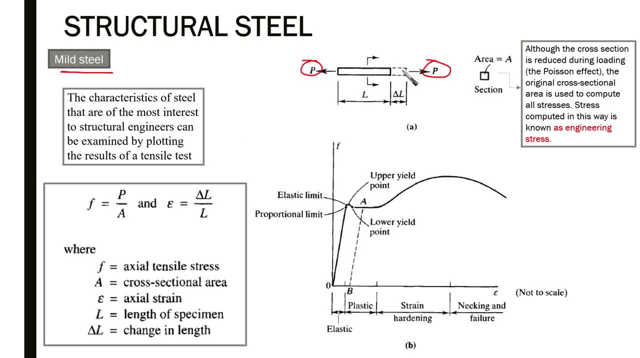 We put it under tensile loading. This specimen is going to elongate. So this relation between the tensile force that is being applied and the strain that is going to be developed, We can plot it here. So we are going to plot the relation between the stress versus strain. 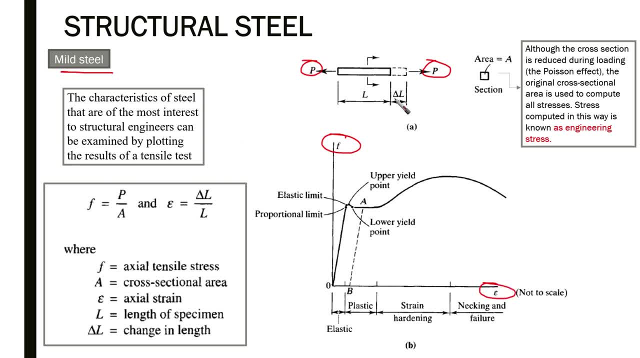 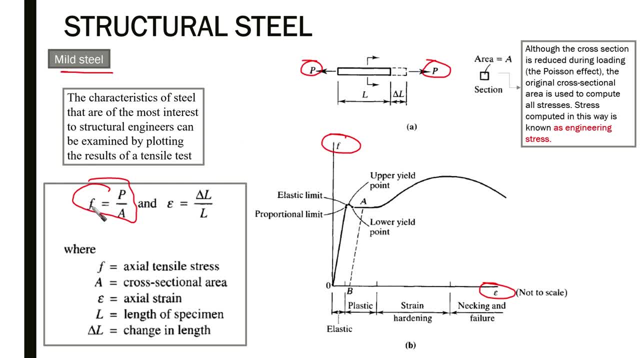 Which is going to be given, as you can see here in this equation F, which is the stress equal to P over A and the horizontal axis, it is going to be the strain which is going to be obtained by dividing delta L, the elongation over the original L. 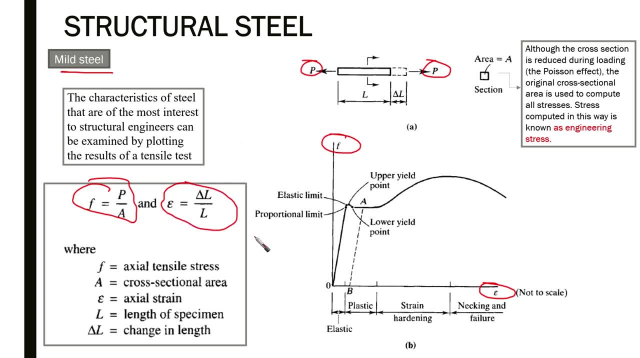 as you can see it here, in this equation, Here, you can see here, I valued this structure as much as the육 ohm proposal And I was going to formulate the Mexican comfortable Tigers, Hahee. So we will have to follow thisstress by multinationals from the sö79, this formula. 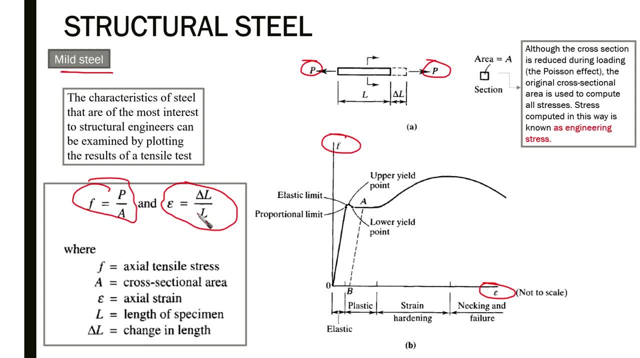 Okay, okay, so everything. now we know about these two equation of the stress and strain, that is: f- we call it the axial tensile stress, okay, and a, it is the cross-sectional area of the bar. this epsilon is axial strain, and l it is the length of the specimen and delta l it is the. 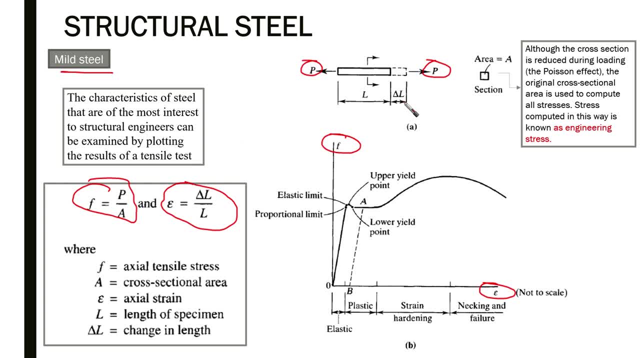 change in the length, as we can see here. we are going to say that this stress, we are going to call it engineering stress. what is the reason for this? actually, because whenever that we are going to apply the force here, the cross-sectional area is going to be reduced. this is due to poisson's. 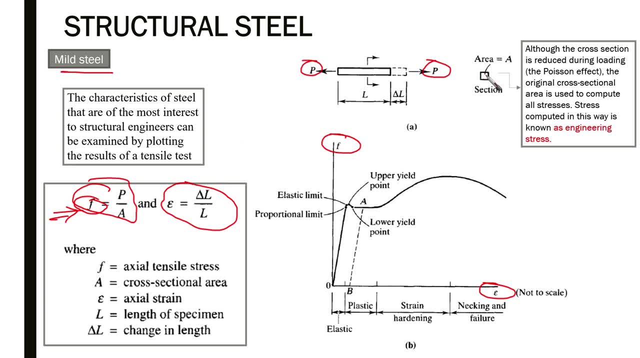 effect. okay, so this cross area, so actually it should be reduced. but actually, as you can see, here we can find that we are using the gross sectional area. so this is why we are not. this is why we are referring to it as the engineering stress. it is not the like actual stress here. so, although the cross-section is, 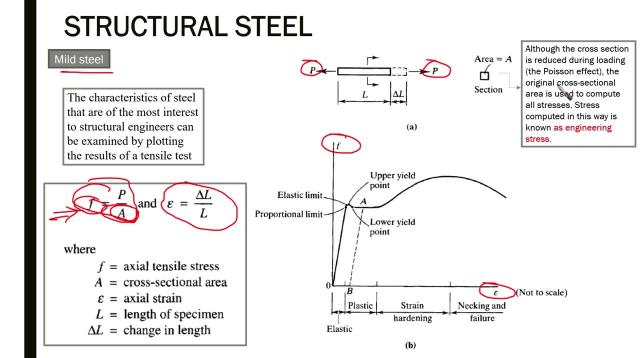 reduced during the loading due to the poisson's effect. the original cross-section area is used to compute all stresses. stress computed in this way is known as engineering stress, so we call this engineering stress. definitely, if you are going to say this is engineering stress, we are. 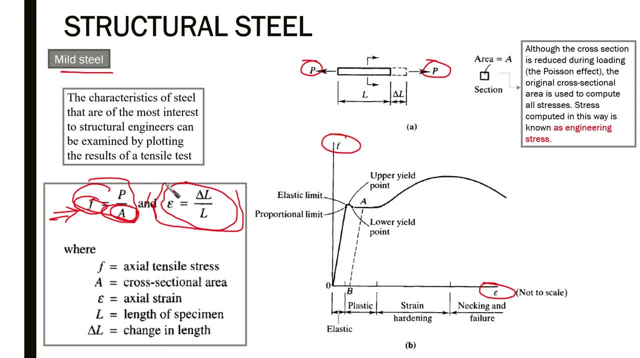 going to call this as the engineering strain. okay, the engineering strain. okay, before jumping to the next slide, we want to look to the stress strain curve for the mild steel. so, as you can see, here, with this bold curve, here, we have different phases for this curve: the first part- we call it the elastic part, we denote it as elastic. 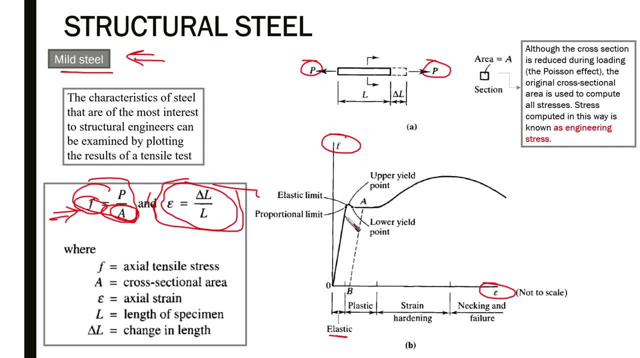 in this part. whenever that we remove the load, okay, the original state of the building is going to be like going to return again, or at least we are going to find that during the unloading phase, the structure is going to follow the same path of the loading phase and this: 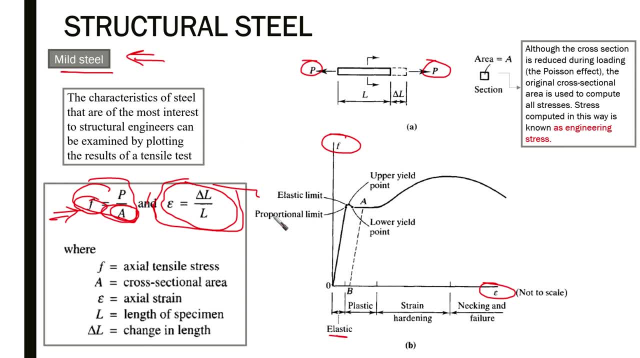 would remain until one point. here we call it proportional limit, and then there is something else called another limit, called elastic limit, and after that the upper yield point, and after that there is a lower yield point. this is the area of yielding here, and after that it is followed by a plateau, as you can see here. 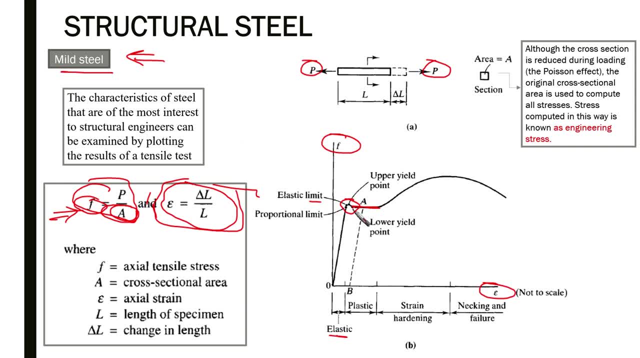 this is we're going to call it the yield of the steel, this area, which is the plateau here, we call it plastic area. plastic area: if there is unloading in this area, you're going to find that this dashed line is going to be the unloading case where that you are going. 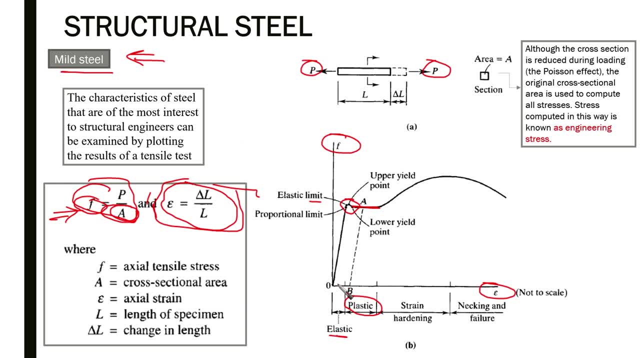 to see there is residual kind of strain, so there is some part that is not going to be used or some part that is going to be considered as residual strain. okay, now let's go to the next part, which is the next phase. we call it the strain hardening, the strain hardening this part. 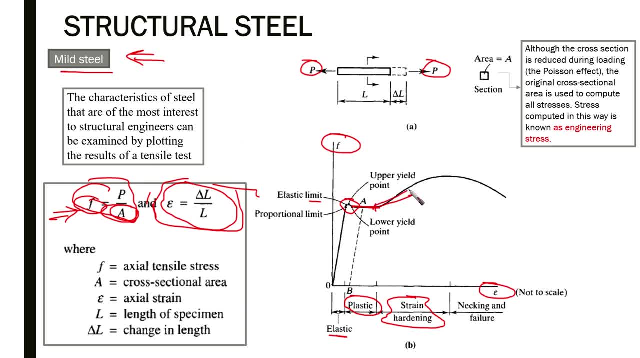 starting from here and going like, as you can see it here, so this part, until here, the strain hardening. you can see this stress is increased, the stress is increased. so the material is showing higher stress, higher than the yield, even until it reaches to a point here which is the start of a phase. we call it nicking and failure. so we're. 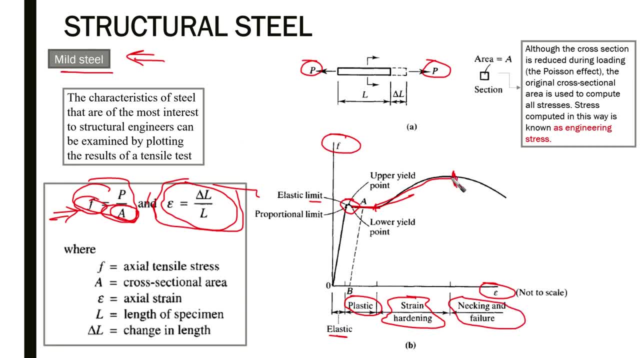 going to find that there is nicking. phase is going to start here in the structure, your or the in this, in this specimen that is nicking here. the cross-section here is going to be highly reduced until that we reach the failure. ok, so this is regarding the mild steel. this is regarding the mild steel. ok now. 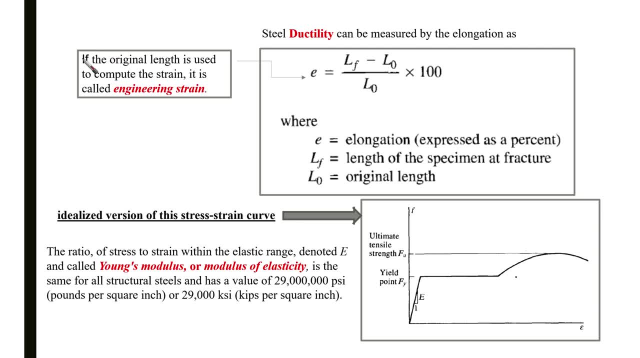 let's go to the next part. as I said, this is the. if the original length is used to compute the strain, it is called the turnover by the body, and that is given by the body. if the original length is used to compute the strain, it is called the. 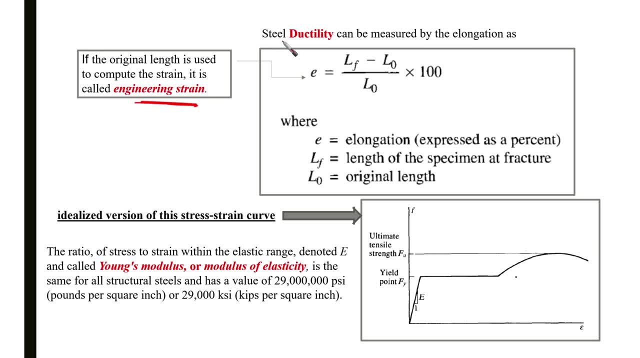 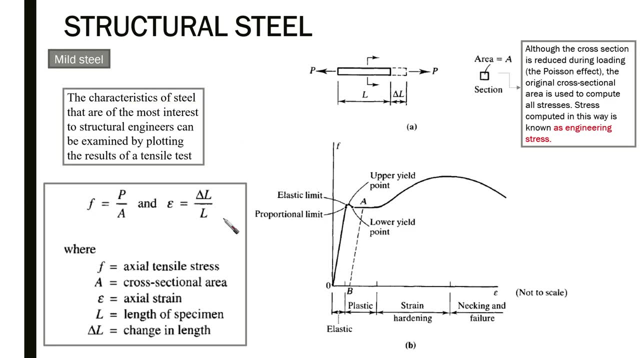 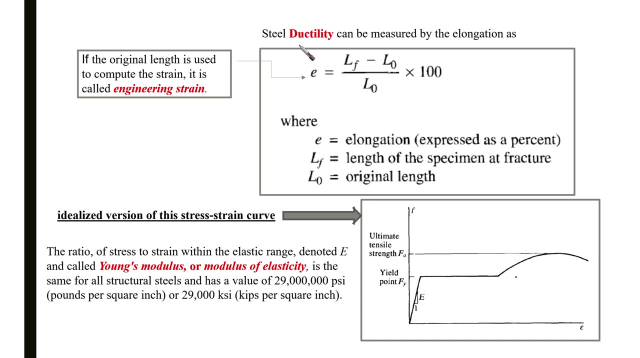 engineering strain. engineering strain- steel ductility- can be measured by the elongation. so actually the engineering strain if we go back here. so this one is going to be the engineering strain, okay, and the steel ductility can be measured by the elongation, as this is we call. 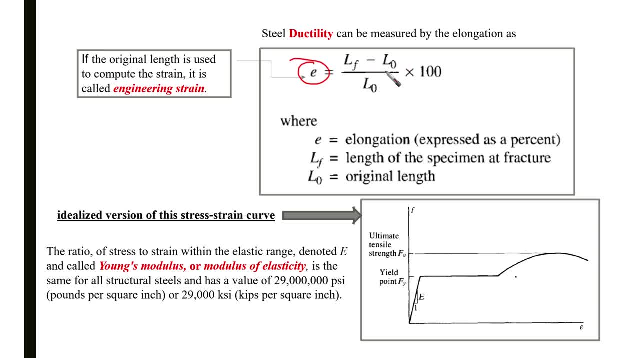 it the steel ductility lf minus l node, over l node times 100, where e it is the elongation expressed as a percent and lf it is the length of the specimen at fracture at the end here, okay, and l node it's the original length if we go back here. so, yes, so all of this distance. 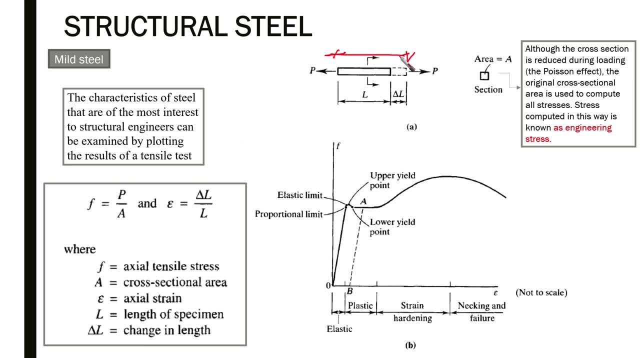 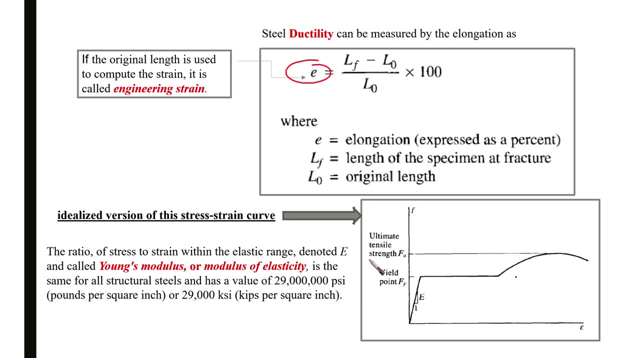 sorry is from here to here. this is lf. okay, the stylus is not helping me, so much sorry for this. and this is of course it is l okay. so this is by which we can up to the steel ductility. okay, sometimes we can idealize the stress string curve in a format that is easy. 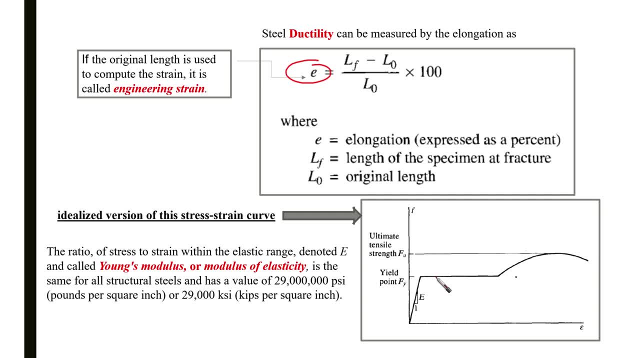 for us to understand and to maintain and to manipulate. so actually we can say that the area or the point that is, there was three points here. we are going to say that it is only one point here and we are going to call it yield. point f: yield and the maximum stress that is going to be reached. 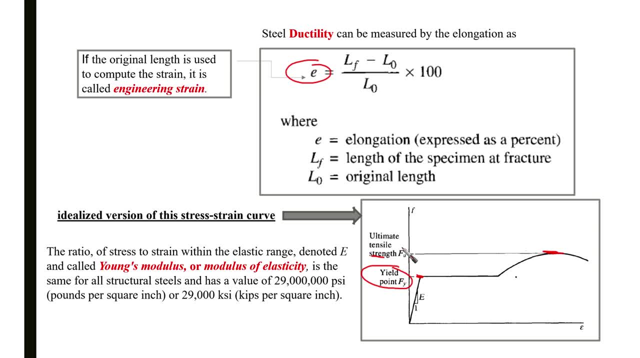 we are going to call it ultimate tensile strength, which is f ultimate. okay, and then we are going to draw it in this way. it's very easy for for us, okay, and then we are going to look to the first portion, which is the elastic portion, and we are going to talk about the, the slope of it. we're going to call: 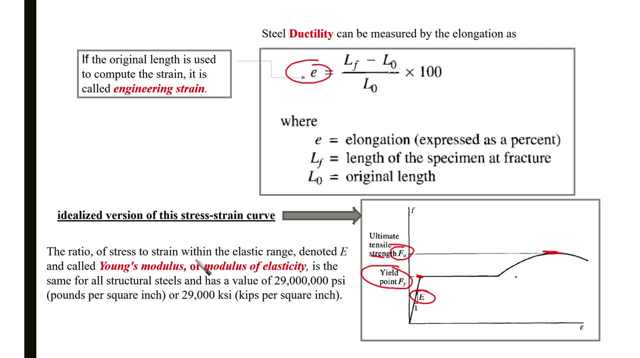 it young's modulus. so the ratio of stress to strain within the elastic range denoted as a and called young's modulus or modulus of elasticity, is the same for all structural steel and has the value of 29 million psi pounds per per square inch, or 29 000 ksi caps per square inch. okay, so this is very. 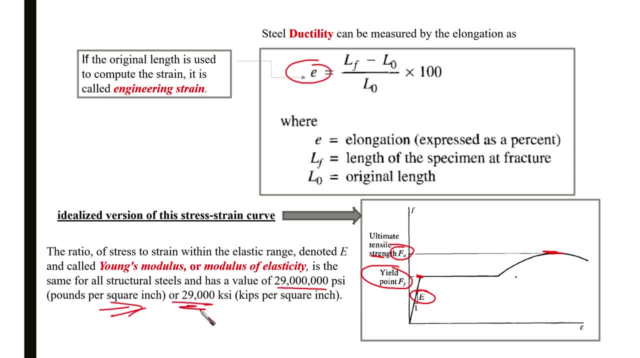 common, remember well, it is constant for all types of steel. there is no difference. we are going to use it for any type of steel, whether it is mild steel or high strength steel or anything else. okay, now we have understood now what are the meaning of mild steel. now let's go to the next part, which is related to the high strength steel. 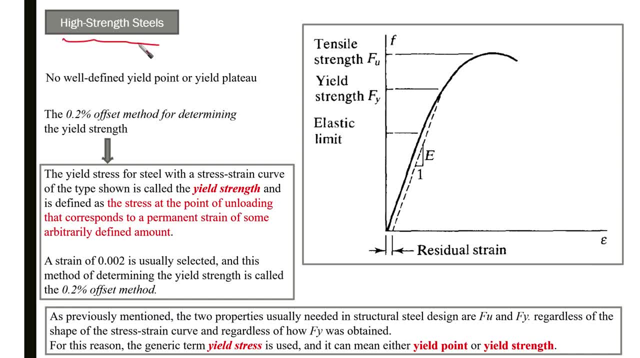 and understand more about it. now let's talk about this high strength steel. as you can see here, the stress string curve is totally different than the mild steel. first of all, you cannot see the plateau and the well-defined yield point. that is something, as you can see, like smoothly making the 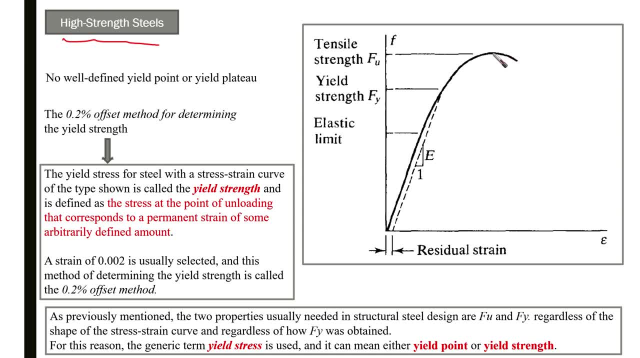 transition between the elastic range to the inelastic range and maximizing the yield point and the maximum tensile strength and the failure after that. it is really smooth here where we can obtain this, so where we can obtain the field. first of all, the most important thing, that is: 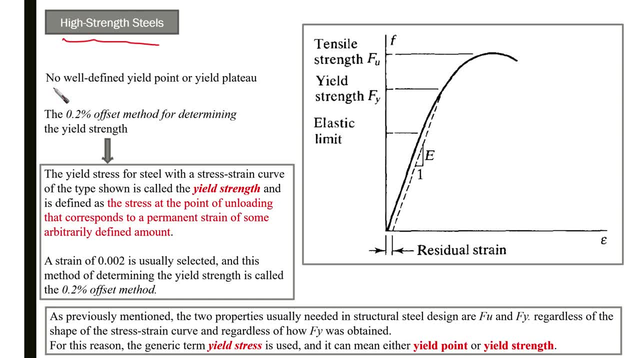 characterizing high strength steel is there is no well-defined yield point or yield plateau. okay, so this is: there is no yield, well-defined yield point or yield plateau. well, how we can obtain the yield, how we can obtain that and say that, this point point here. then there is a method called the 0.2% offset method for determining. 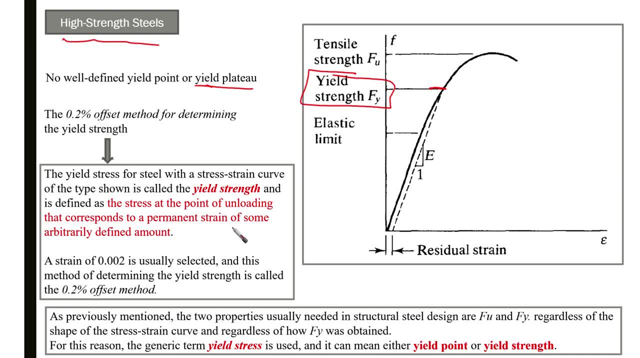 the yield strength. so actually we are the yield stress for steel, with the stress-strength curve of the type shown is called yield strength and is defined at the stress of the point unloading. that corresponds to a permanent strain of some arbitrarily defined amount. so here we are going to come at the strain. 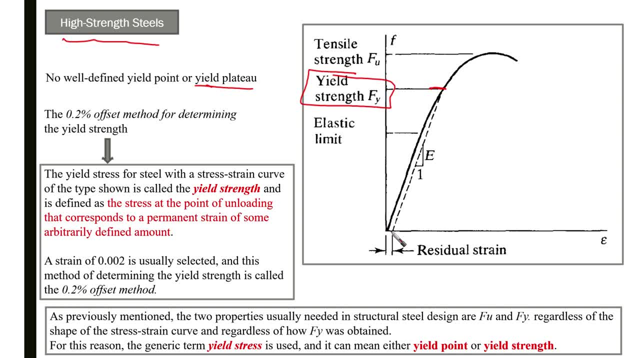 axis and we are going to measure 0.2% and then we're going to draw this dashed line parallel to the elastic range. this dashed line is going to intersect the original curve at a point. this point we are going to call it exactly, we are. 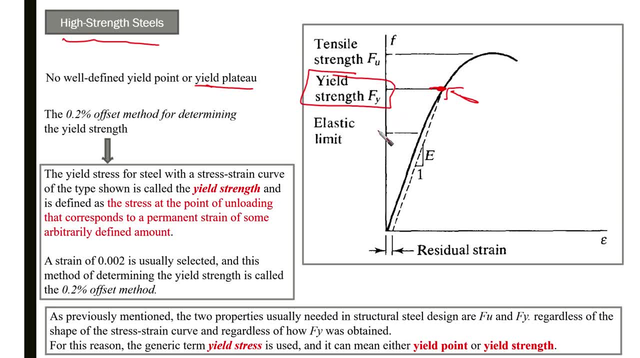 going to call it the yield strength of this material. okay, okay, a strain of 0.002 is usually selected, and this method of determining the yield strength is called 0.2% offset method. okay, so that's how we can obtain the yield. the yield strength regarding the 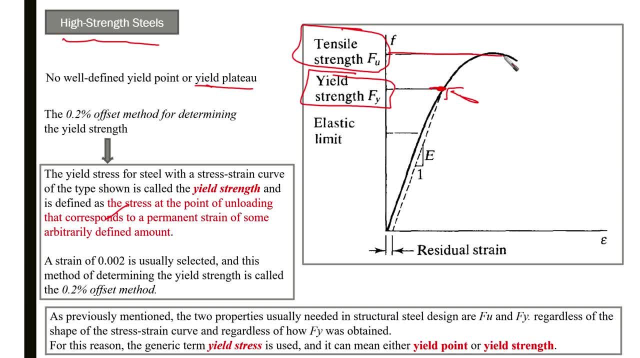 tensile strength, which is F ultimate. it is very easy because the maximum value here it is going to be F ultimate. as previously mentioned, the two properties usually needed in a structure steel design are F ultimate and a field right. we said that they are the most important. 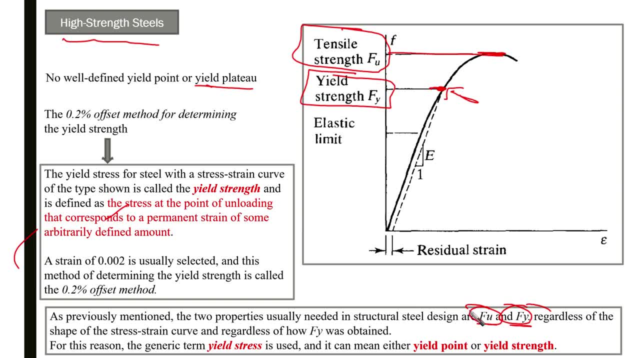 two properties, the most important properties, that is, you are going to find that we are going to use them in everything. almost in every design example. we are going to use one of them, or both at least, regardless of the shape of the stress turn curve and regardless of how F yield was obtained. so always. 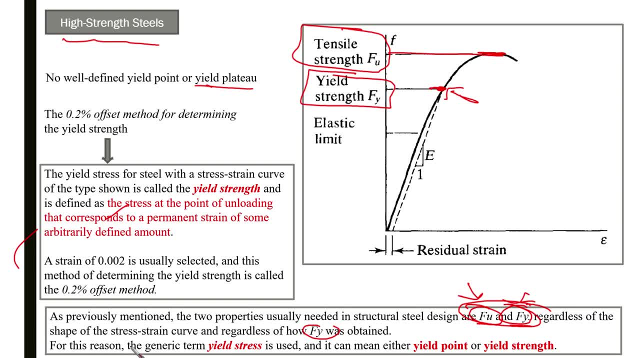 we are going to use F- ultimate and F- field. for this reason the generic term yield stress is used and it can mean either yield point or yield strength, so they are like interchangeable. you can say yield stress or yield strength, okay, so they are. or the yield point, all of them. 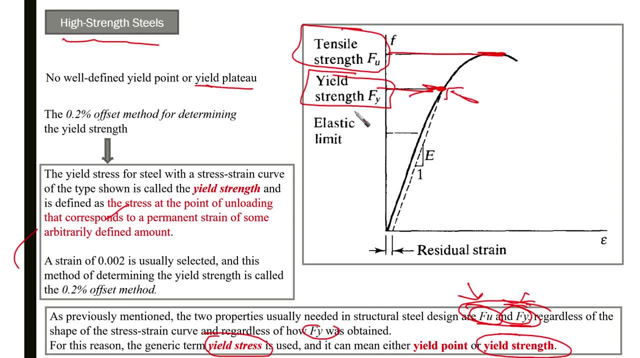 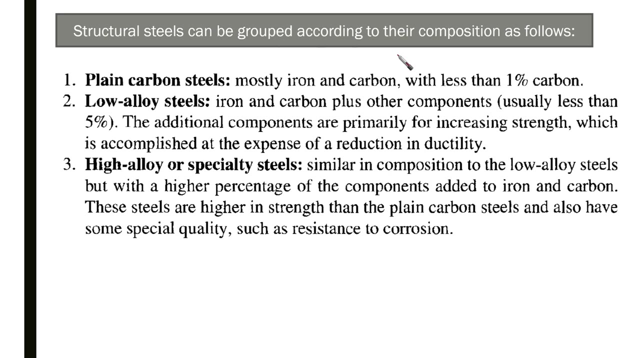 they are like making the designation of this yield strength F field. okay, now let's go next. after that work, we need to go and know about the structure steels and how we can group them based on the composition. okay, let's go to the next slide. yes, we have structural steels that can be grouped. 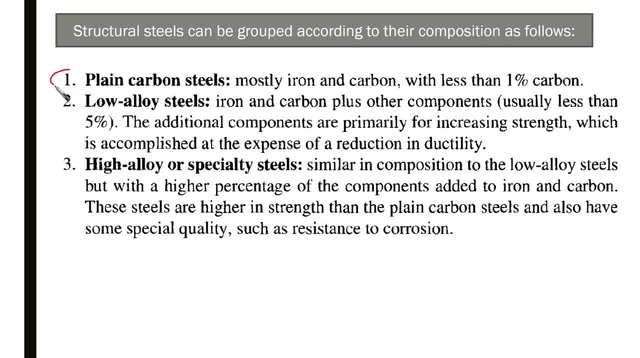 according to their composition, as follows. we have three main groups that we can categorize the steel based on which the first one is. the first one is the plain carbon steels, mostly iron and carbon, with less than 1% carbon. okay, this is the first one, which is the mild steel, always belonging to 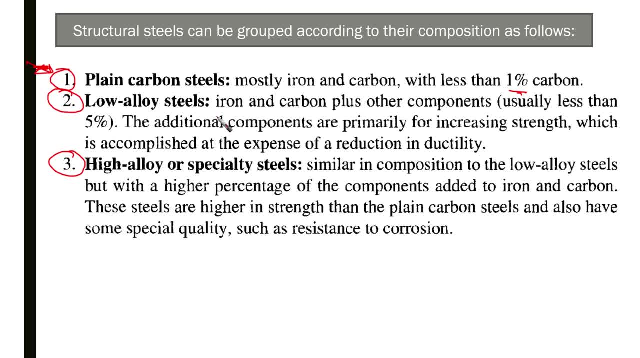 okay. and number two: it is low alloy steels, iron and carbon plus other components, usually less than 5%. the other components are always less than 5%. the additional components are primarily for increasing strength. that's the point here. we are increasing the strength by adding additional components. 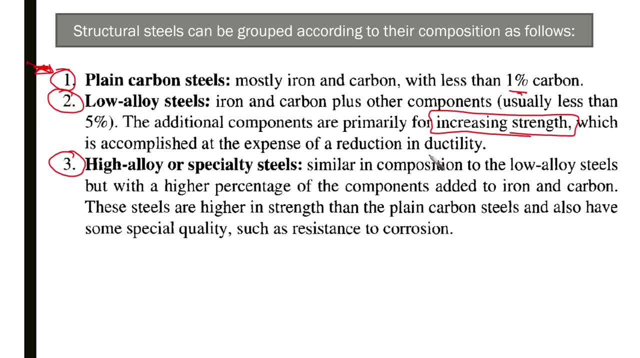 which is accomplished at the expense of reduction and ductility. so whenever that we are adding additional components for increasing the strength, it is always at the cost of ductility. so there is a trade-off here. and the third one is going to be high alloy or specific, or 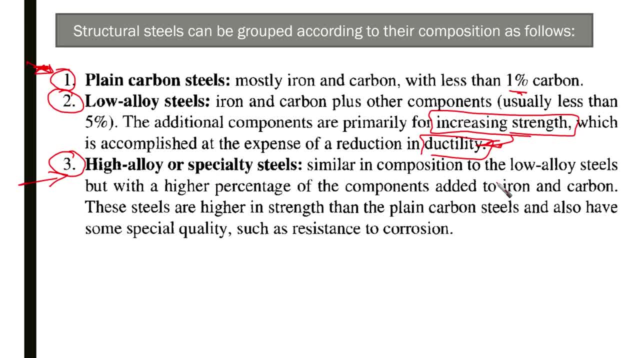 speciality steels. it is similar in composition to the low alloy steel, but with a higher percentage of the components added to iron and carbon. these steels are higher in strength, so they are maintaining the higher strength, as we always need. then the plain carbon steels, which are high in strength, as we always need. then the plain. 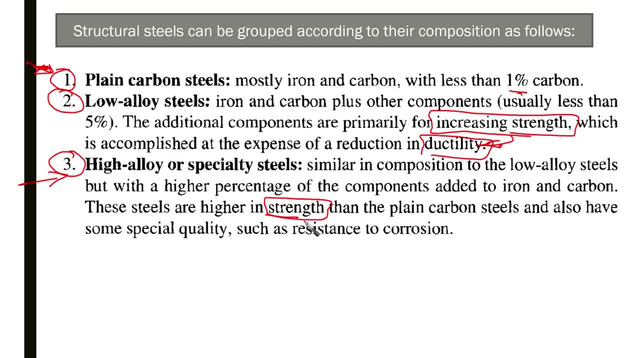 carbon steels, which is group number one, and also have some special quality, such as resistance to corrosion. so this is one of the main qualities that we can obtain using high alloy or speciality steels. okay, so we can group our our structure steel into these three groups, okay. okay, now let's go to the next slide. 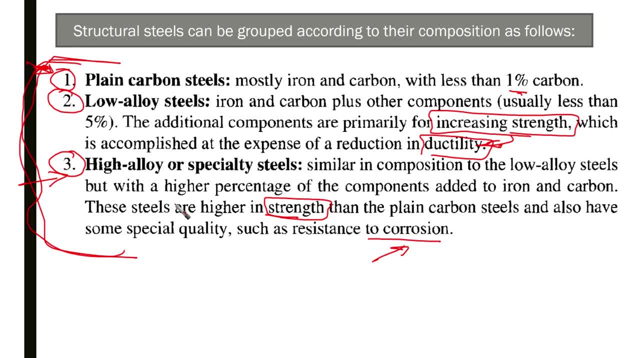 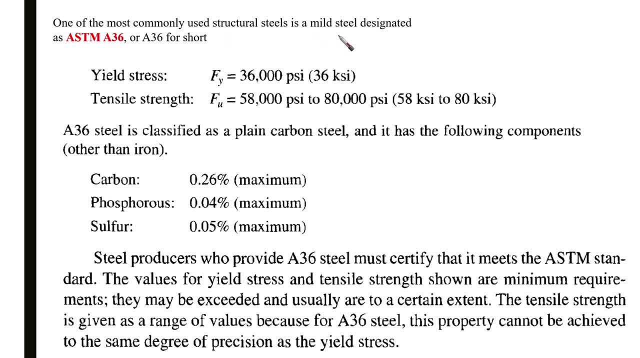 which is related to one of the most commonly used steels. its go. so here. one of the most commonly used structure steels is mild steel designated as ASTM or of ASTM A-36 for short. this is one of the most common commonly used structure steel and its yield stress, I feel it is 36 thousand psi or 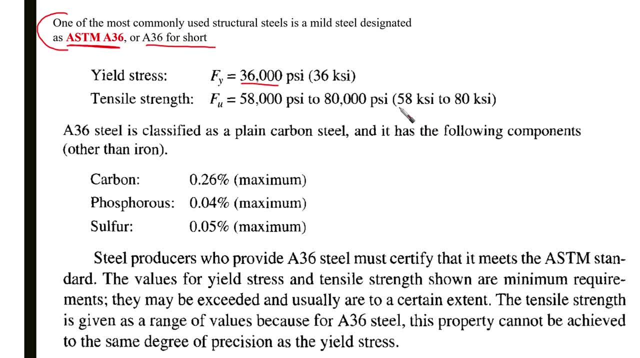 36 ksi and its internal PCM is over 3 temp of Mercedes, or in other words, interface Silic strength ranges between 58 KSI to 80 KSI. okay, So this is. you need to remember them well and you need to memorize them well. 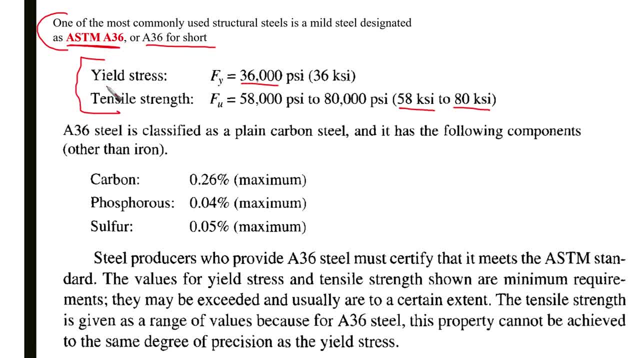 because almost in many of our examples, we are going to use it. okay, A36 steel is classified as a plain carbon steel, So it is from category number one, as we discussed in the previous slide, and it has the following components: 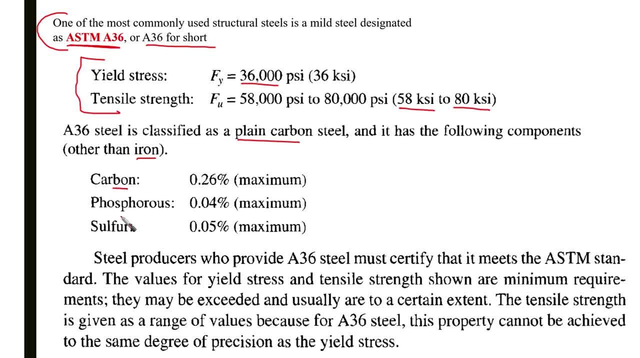 other than iron. of course, It has carbon, phosphorus and sulfur. with these percentages here, okay, This is maximum means that we can get more or we can add- sorry, less than this. This is the maximum to be 0.26%. 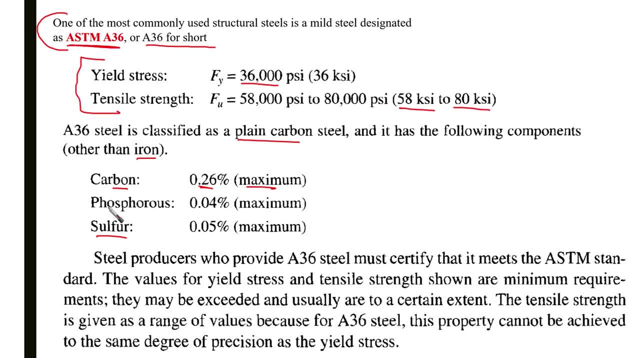 We can add less than this value, Similar to phosphorus, which is like 0.04% maximum, and sulfur, 0.05% maximum. Steel producers who provide A36 steel must certainly be aware of the fact that it meets ASTM standards. 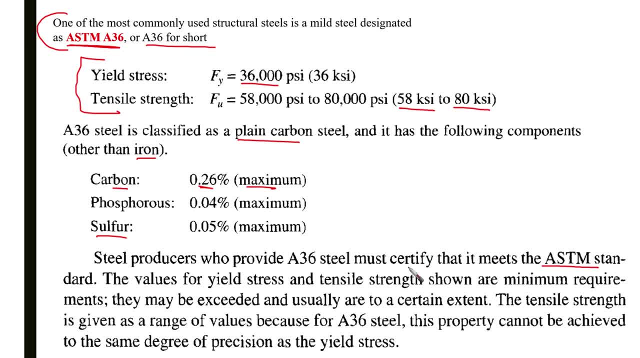 So whenever that you are going to design your steel structure, you need to always have a certification from the steel provider that it meets the ASTM standard. The values for yield, stress and tensile strength shown are minimum. That's very important. It is minimum requirements. 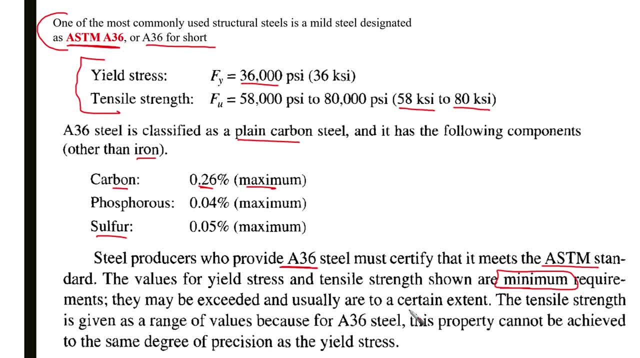 They may be exceeded, and usually are to a certain extent. This means that this 36, it is the minimum. Actually, in reality, you're going to find that the yield stress is higher than that- And also for tensile strength, this is the minimum. 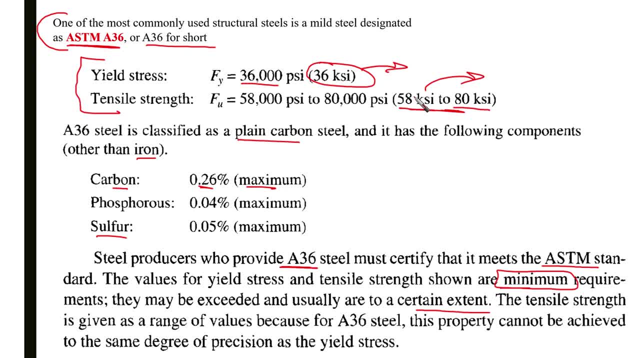 You can find that in reality, the tensile strength is higher than the value that you used in the design. okay, And this is why the overstrength is always coming from. So we do not know exactly what is the yield stress, the actual yield stress in our 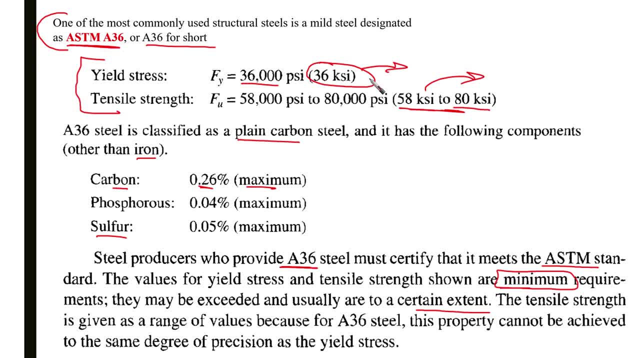 used in our members and components, Whether that we use 36, but actually maybe it is larger than this, Maybe it is 40. Who knows about this? From here, we can say that there is overstrength in this point and we can like have more overstrength factor in our design. 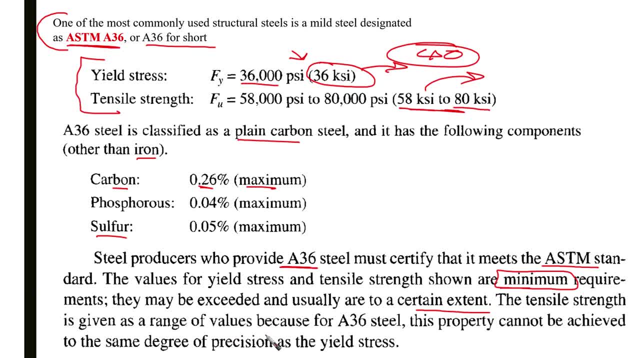 Anyway, the tensile strength is given as a range of values, because for A36, as you can see here, this is a field- it is given as specific value. However, for the tensile strength it is a range. What is the reason for this? 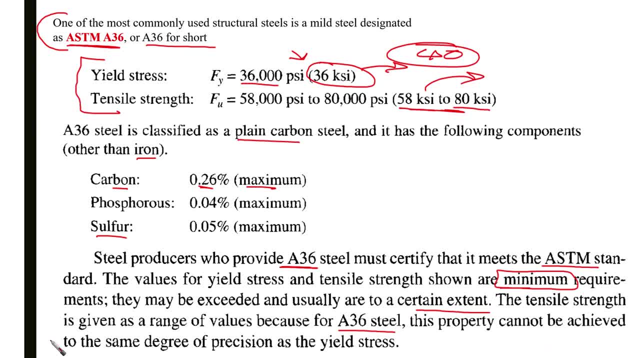 Because this tensile strength cannot be achieved to the same degree of precision as the yield stress. We cannot, based on the experiments and so on, we cannot get the accuracy of the yield stress, as we, whenever that we are measuring the tensile strength. 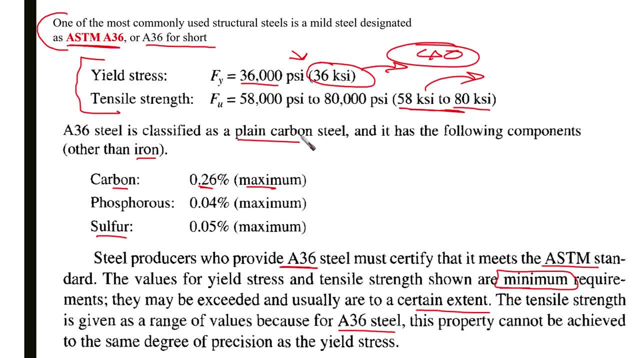 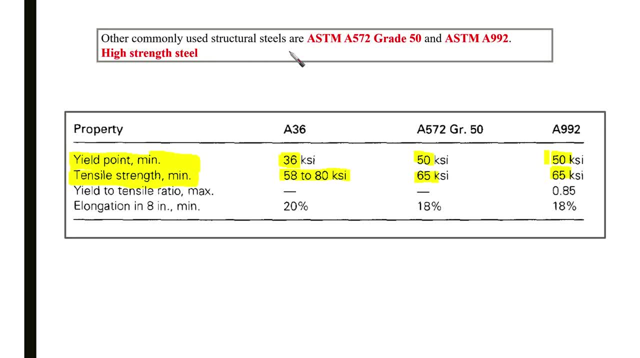 Okay, Okay, now let's jump to the next slide to see what are other types of steel that we can use in our design. So other commonly used structural steels are ASTM A572, grade 50, and ASTM A992.. They are the two major high strength steels. 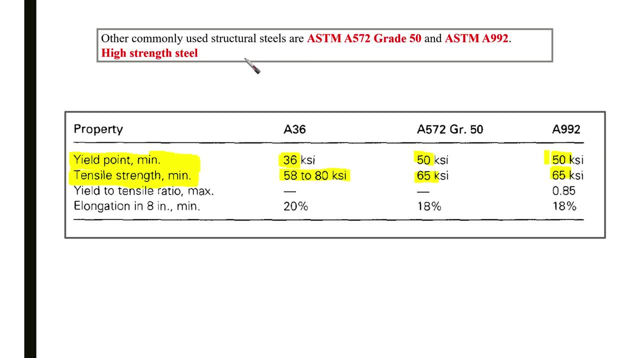 or common high strength steel, structural steel that is being used, And we call them high strength steel. So, anyway, now for the most common structural steels that we are going to use in this course. we are going to focus on these three ones. 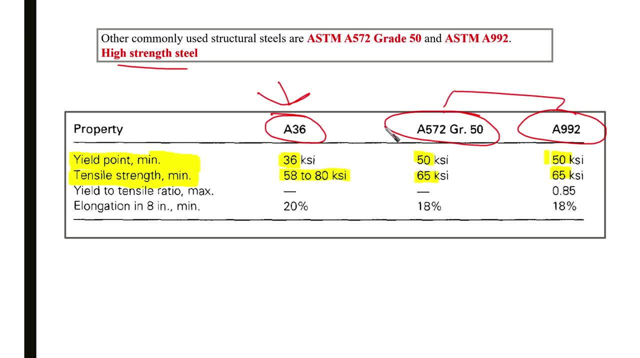 This is mild and these two are going to be high strength. The minimum yield point for A36, it is 36. And tensile strength ranges between 58 to 80.. For A572, the yield point minimum is 50, similar to A992.. 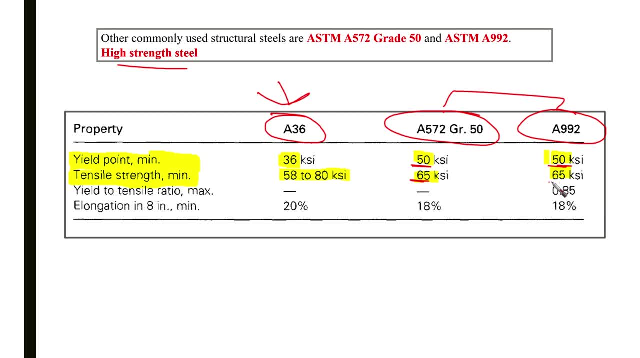 And the tensile strength. it is 65, similar also to A992.. Okay, So this is like the major and the most important properties that we need to use. Let's go and see what is the typical stress string curves for similar or for these kinds of steel in the next slide. 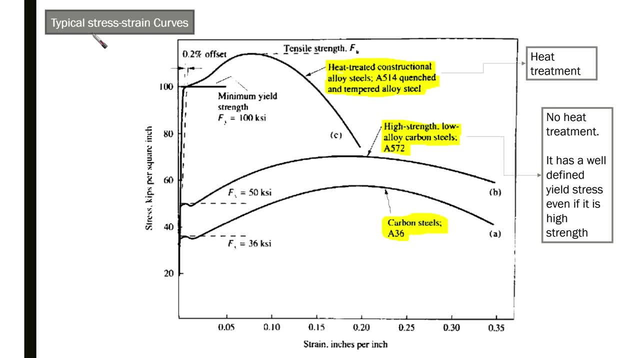 So this is the typical stress string curve. This is the typical stress string curve, as you can see. So in the horizontal axis it is the strain, vertical axis, It is the stress in kips per square inch. And here, the first one here, which is this curve: 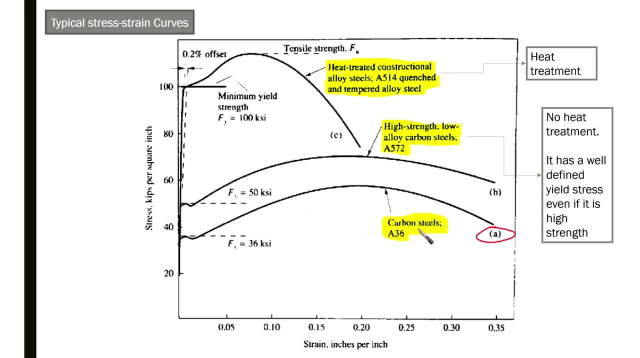 which is curve A. it is the carbon steels, which is like A36,, for example, as you can see here, This is the yield. F yield is 36 ksi. The curve B, as you can see it here, this is the high strength, low alloy carbon steels. 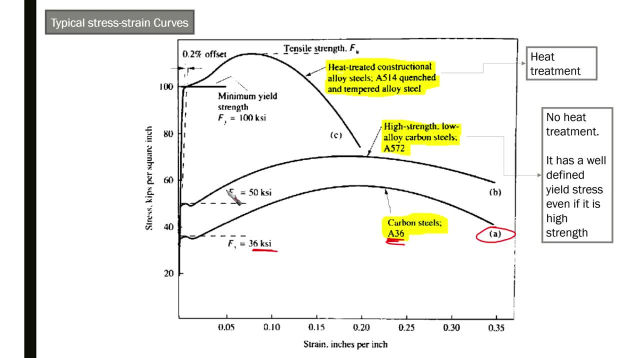 A572,. as you can see, It is having like higher strengths and the yield is higher as well. okay, So it is. maybe you are going to ask that. we said before that for high strengths it is not well-defined here. 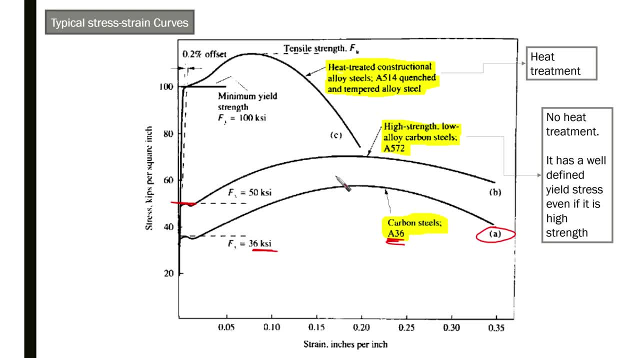 Actually the yield should not be well-defined, but actually for this type of high strength steel- okay, high strengths with low alloy carbon steels, this type of steels, because it is- it has no heat treatment. It has no heat treatment. 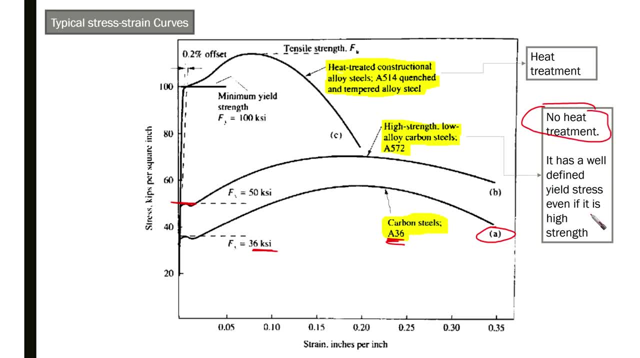 So it has a well-defined yield stress, even if it is high strength steels, okay. So this is like, because of the way of production itself, it can be provided with, or at least it can give us a very well-defined F yield. 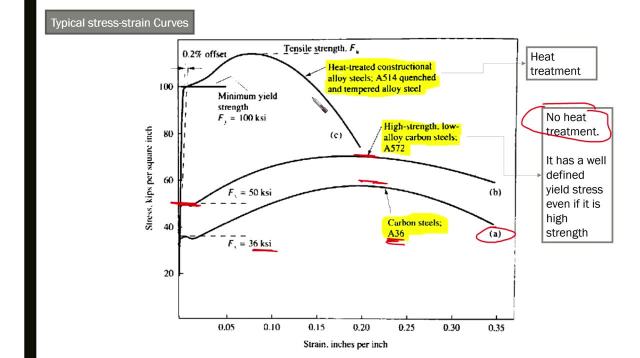 and higher strengths than the mild steel. This one. it is considered to be the real high strength steel, which is: we do not know exactly where is the F yield, but we can be sure that it is high strength steel. But if it is high strength, 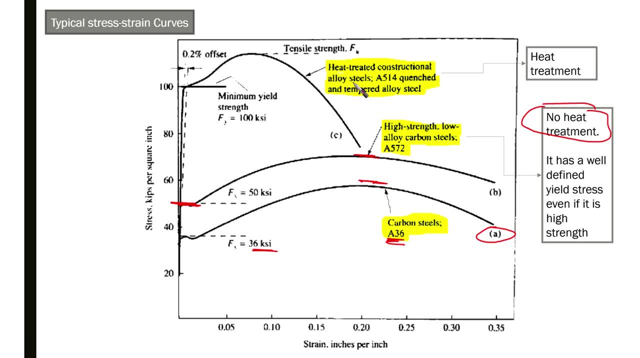 it is a very, very, very high strength of steel. We call this a heat-treated construction constructional alloy steels. A514, quenched and tempered alloy steel. This is heat treatment, So we're going to find it is very high here. 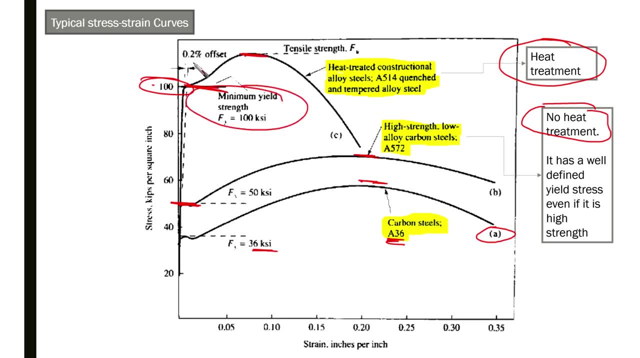 The yield is almost like around 100, minimum yield strengths around 100. And the strengths here it is very high also compared to these kind of steels that we are talking about And we are going to know here and we are going to. 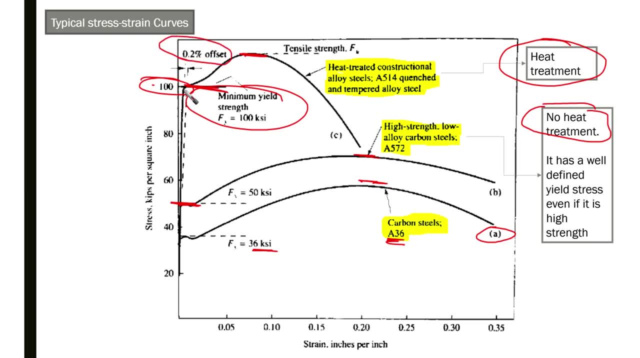 going to use the 0.2 percent offset strategy or scheme in order to obtain the yield here. okay, so this is the typical stress string curves for different types of steel. now let's go to the last part of our course for our video for today, which is the standard cross-sectional shapes. 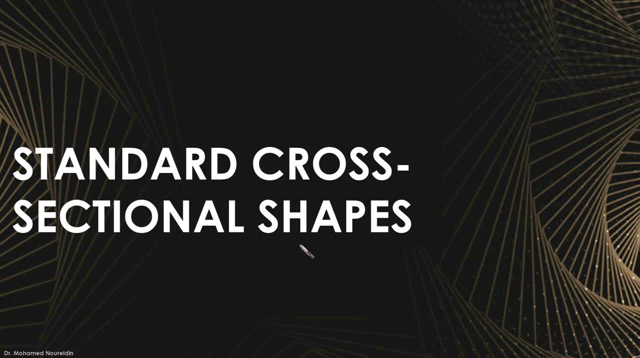 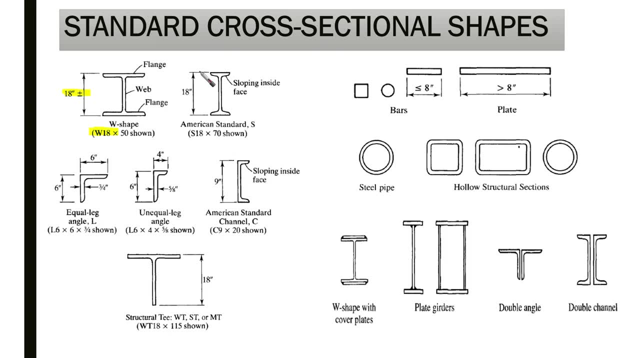 yes, so we're going to talk about the standard cross-sectional shapes that we are going to use in our examples and applications. so actually we have standard cross-sectional shapes here. we have different shapes. we are going to refer to them, so you need to be familiar with them before. 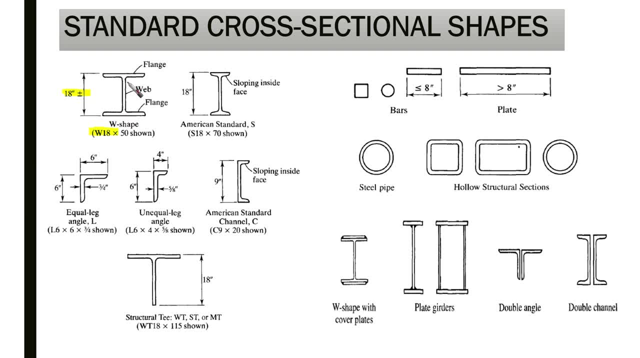 starting the course. commonly we are going to use what we call it the wide shape or wide flange. as you can see, here the flanges are a little bit wider compared to the american standards that we are using commonly. so the wide flange. you're going to find that the flanges are a little bit. 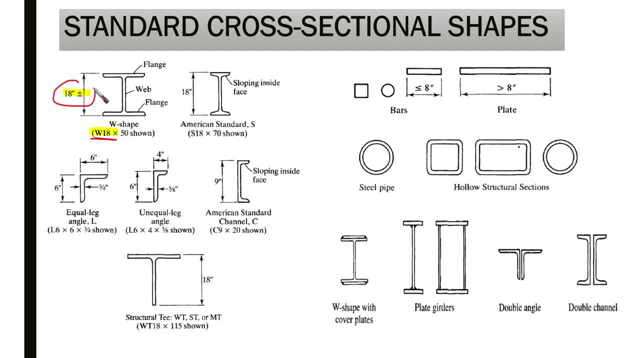 uh, here w18. this means that the height of this cross section is plus or minus 18 inches and the uh, this is the weight per unit, uh length of it. we call it the wide shape. this is the web, this is the two flanges here, and then we are going. we, we have also another type of standard. 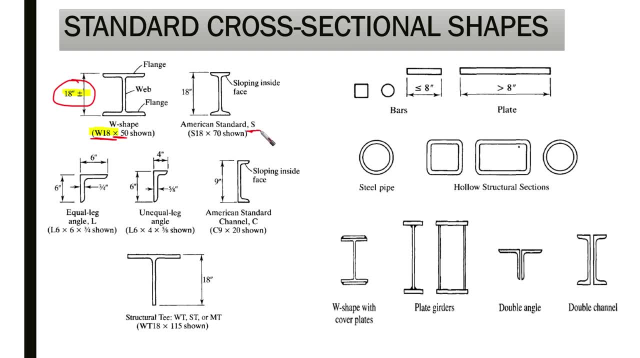 cross-section. we call it american standard, which is denoted by s here. this one is denoted by w- s18, by 70, for example. this is the height also is 18 inches and we have sloping inside face, as you can see it here. then we have equal leg angles, as you. 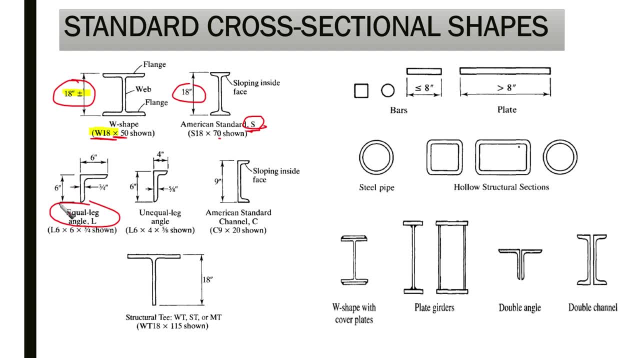 can see it here with: the two legs are equal and the thickness is going to be given. so this is l6 by 6, by 3 over 4, means that the equal length for the two legs and the thickness is the same. okay, and after that unequal leg, as you can see, one leg is shorter than the other and the thickness 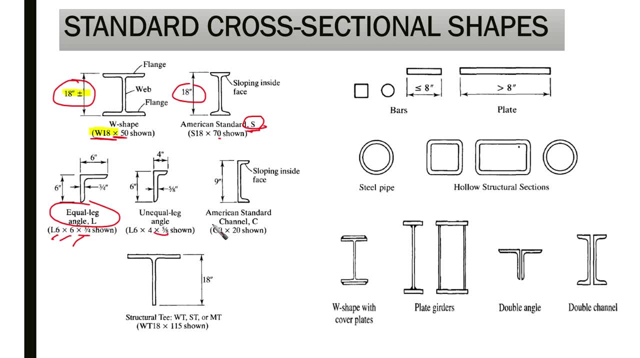 is given here. it is the same for both legs. this is what we call it, the angle. and then we have this one which is the american standard channel. okay, we call it c9 by 20.. so nine means that the height of the channel 20. it is the weight per unit length, similar to 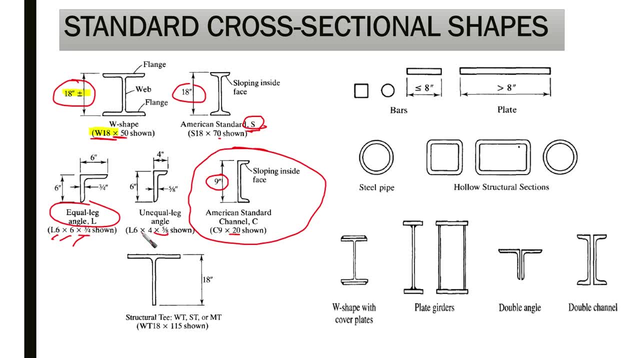 the wide flange and the standard, american standard, and then we have the t and the structural t, which is wt. t means that it's cut from a wide flange, or s t cut from the longer flange, from the length and the middle flange, which is the�. and then we have the, so it's the body sheet voucher. rug called the DUI, which is the width of your body, and so you cut the width of your body out by moving that into right andiod. so this is what we're doing: we're doing it to this yellow outer part and now open, here we have the tambéอ, in the right, most white angle, epsilon, which is to put aOR on the goddess. 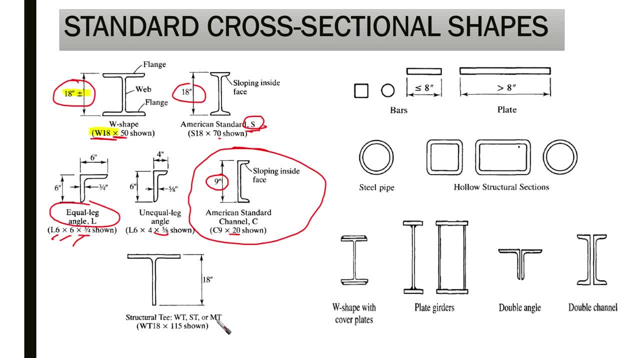 or st cut from the american standard, or mt miscellaneous. it means that it is not w, not s, it's miscellaneous cross section and it has been cut to bt. wt, for example, means 18- the height is 18 inches, as you can see- and the second one is the weight per unit length. we have bars, as you can see. 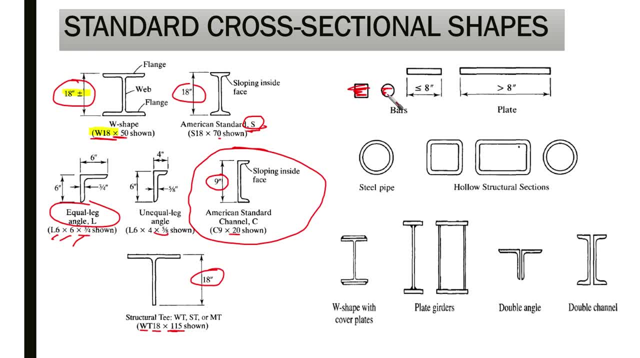 which is, as you can see- this is the bars here- which is solid from inside. we have plates which should be larger. the width of the plate should be larger than eight inch, but if it is less than eight inches, then it we call it bar. we have steel pipe, as you can see here, hollow from inside, and it. 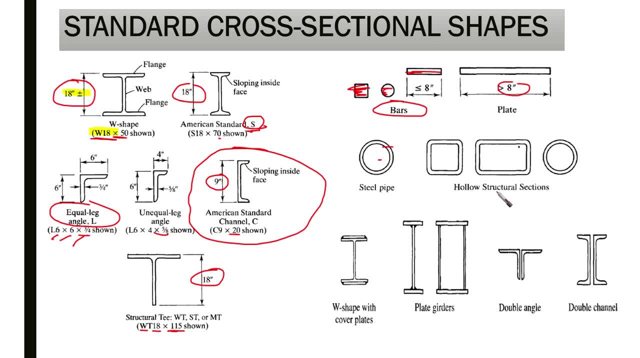 has a thickness. we have hollow structure steels, or, sorry, hollow structure sections, which means that it is going to be, as you can see here, whether it is square or rectangle or or hollow structure steel in shape of a pipe similar to the bike. okay, but we have like standard sections for steel pipe and we have another standard section for hollow structure steel sections for the circular shape. then we have another types, which is like plate girders, coming from built up sections, wide flange with cover plates. as you can see, we add some cover plates and the top and bottom flanges. we have plate girders here, which is going to be a 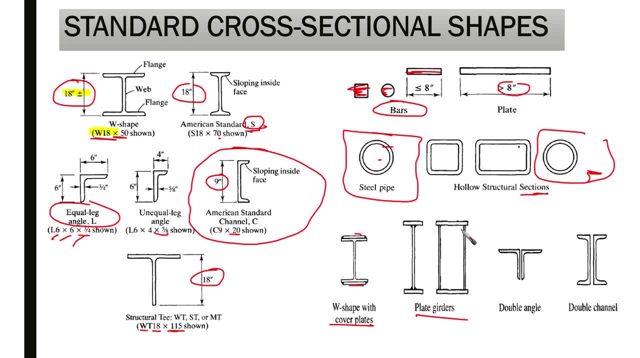 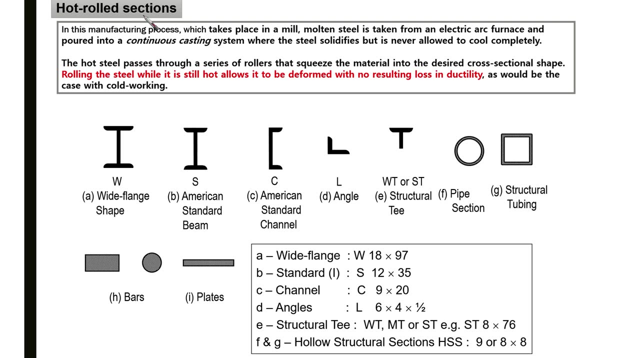 composed of the web is going to be doubled. for example, double angle- we put them back to back. or double channel- two channels back to back. okay, we have two types of sections commonly used and commonly mentioned, which is hot rolled sections, and we have cold rolls, cold formed sections. for the hot rolled. 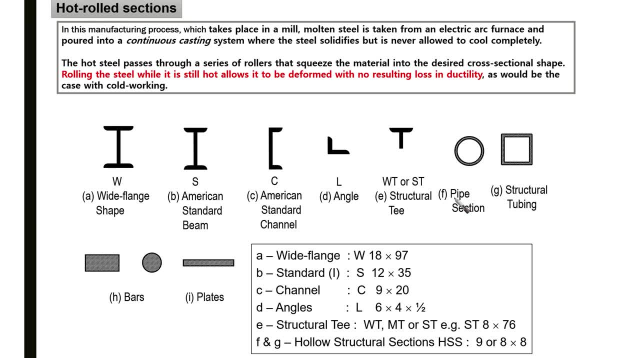 sections generally. these are the hot rolled sections, as you can see all of them we have explained about, about, out, about, about about them: the white flange, american standard, american standard channel, the angle, or the t's section, pipe section, structural tubing, bars, plates, all of them, they are hot rolled. what is the meaning of? 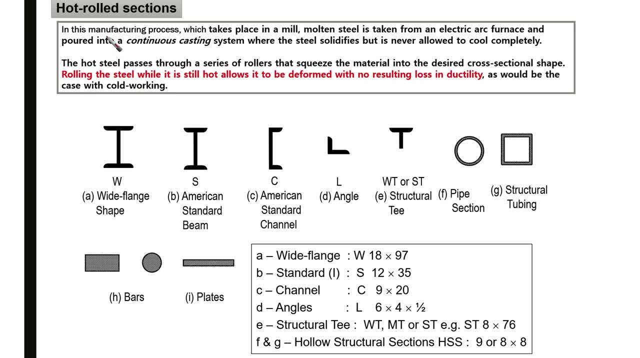 hot rolled actually it is. basically it is related to the manufacturing process and the hot rolled manufacturing process. it takes place in in a mill. molten steel is taken from an electric arc furnace and poured into a continuous casting system where the steel solidifies but is never. 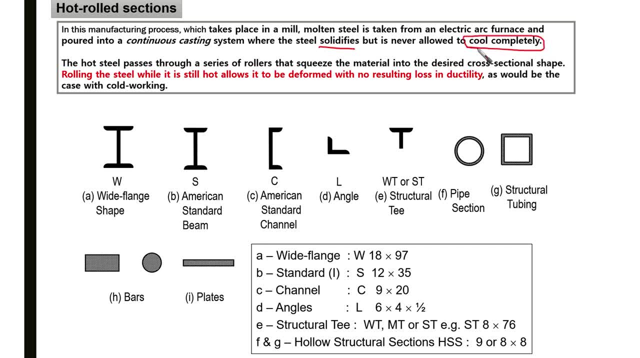 allowed to cool completely. that's the that's the key here. it is never allowed to cool completely. the hot steel passes through a series of rollers that squeeze the material into the desired cross-sectional shape. rolling the steel while it is still hot allows it to be deformed. 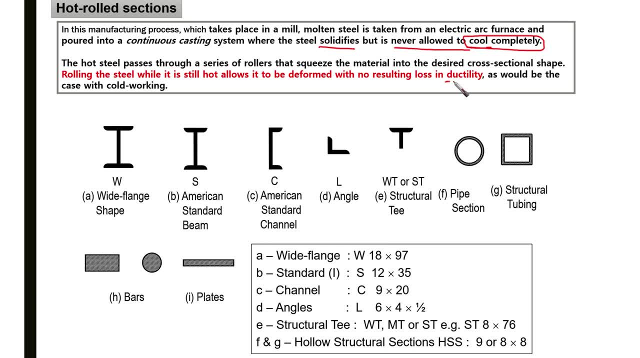 deformed. deformed with no resulting loss in ductility. that's is another key that you need to remember whenever that we mentioned about hot rolled. so the process itself, the process itself, it is the manufacturing process it is. the point is, we are like pouring the molten steel. okay, taken from. 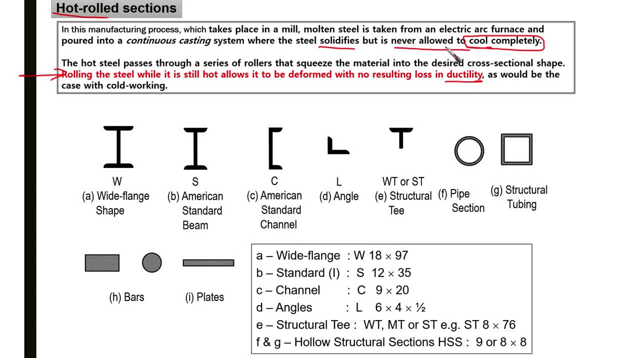 the electric arc furnace and we put it in a casting system, but we never allow it to to cool completely and then we can deform. okay, so there are some rollers, series of furlers. they are going to provide the desired cross-section that we want. but rolling the steel while it is hot. 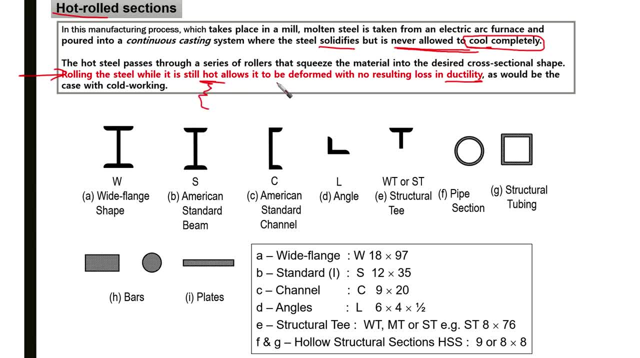 that's the point here. it is hot, allows it to be deformed with no resulting loss and ductility. that's the main advantage it is in in comparison with or in contrast with the cold formed, as would be the case with cold for cold formed, all right. so let's go ahead and go ahead and actually let's. 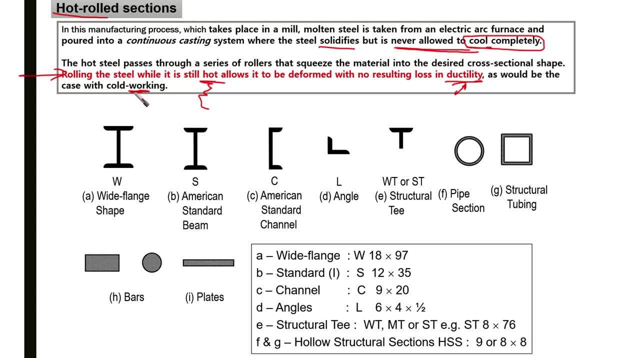 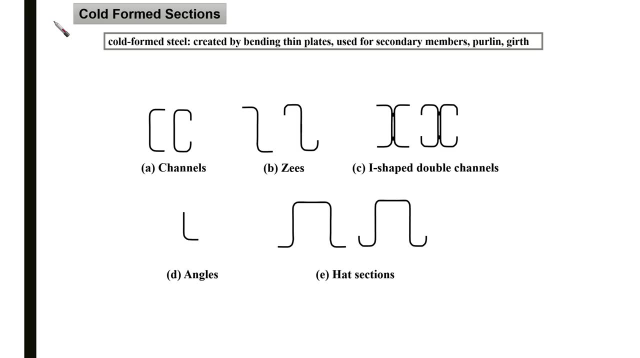 Cold working. no, it is cold formed or the cold formed sections. it is different than this. We are not shaving it while the material is hot. This is not the case if we are going to talk about the cold formed, as we are going to talk here. 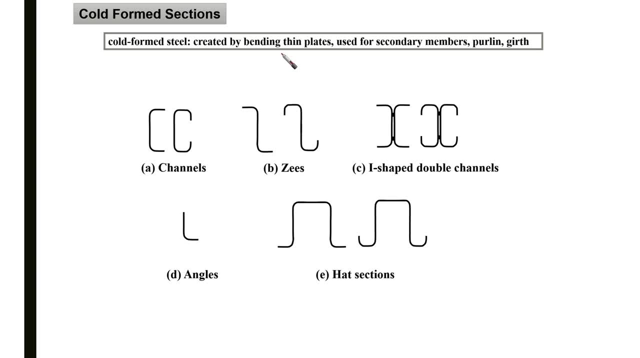 So the cold formed steel created by bending thin plates used for secondary members- perlin and girth- and it is using the cold steel, not hot trawled steel. These are common shapes that is being used for the cold formed channels, These I-shaped double channels, angles and head sections. they are commonly used for secondary members. 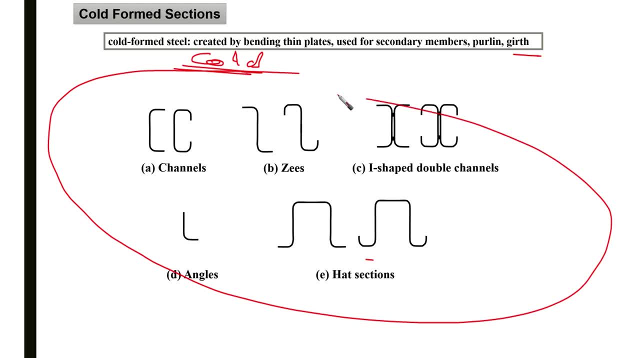 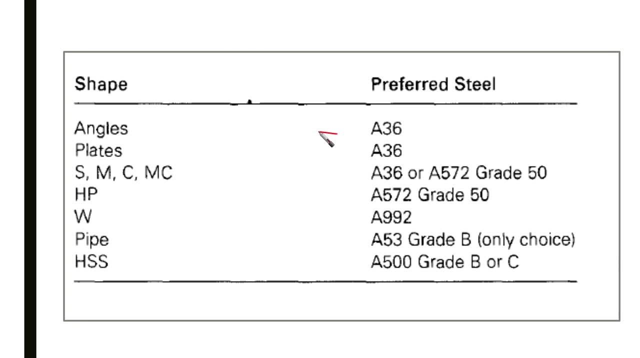 We are not going to use them and study them in our course. okay, It's only for information. The last slide maybe is going to be about what is the preferred type of steel that is used for every shape. So for angles and plates, A36 is commonly the main preferred steel material. 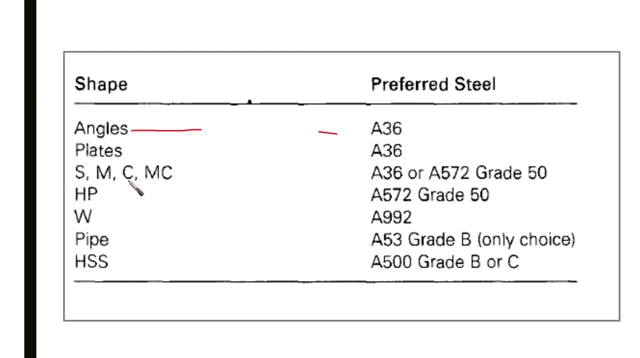 For American Standard for miscellaneous for channels. for miscellaneous of channels, we are commonly find them in A36 or A572 grid 50. HPs: they are going to be A572, grid 50. Wide flanges. commonly they are high strength steels.